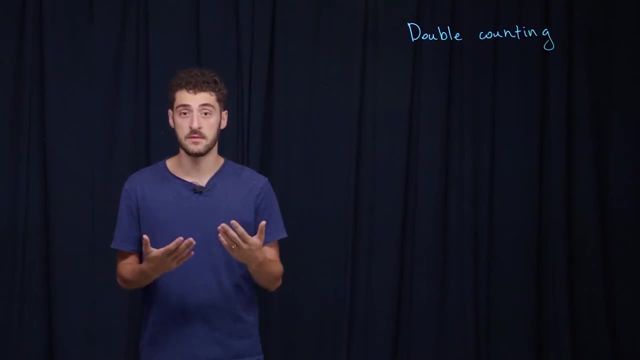 matter how you compute the size, the number should be always the same, And double counting is based on the idea that you count the size of a set twice and you get an equality. Let's illustrate this using the following example. Let's imagine you are in the party and there. 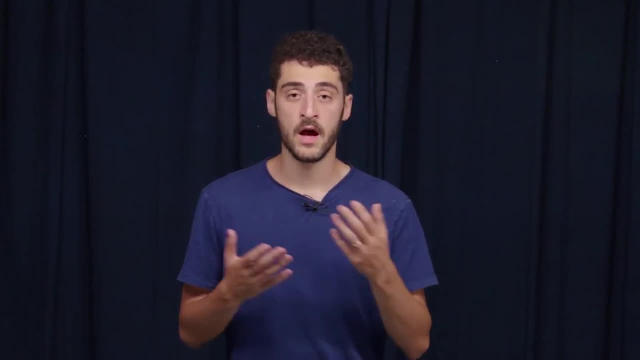 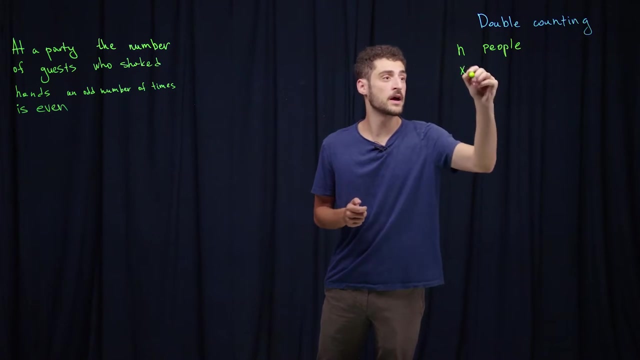 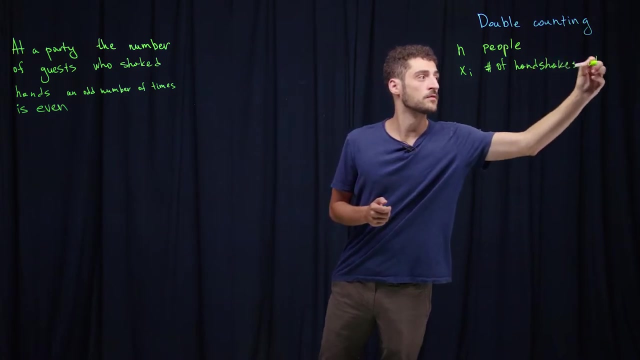 are several people there. they're handshaking each other And the claim we are going to prove is that the number of people who handshake odd times is even. Let's try to prove this statement. Imagine that we have n people and xi be the number of handshakes of the if-person. 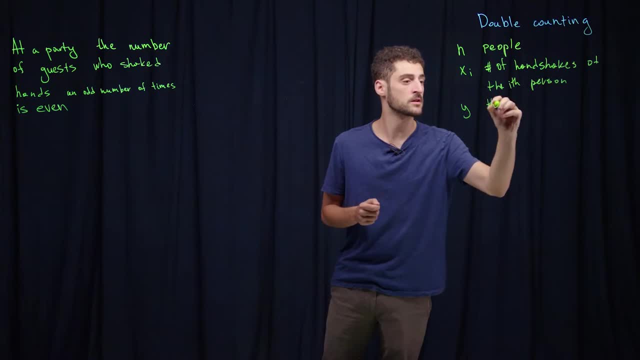 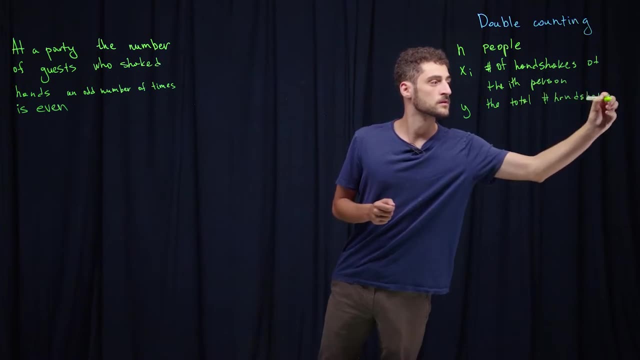 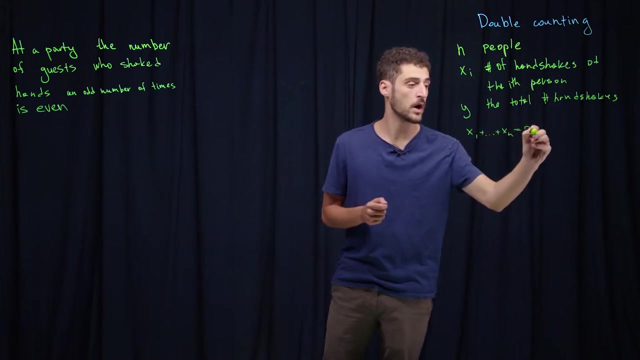 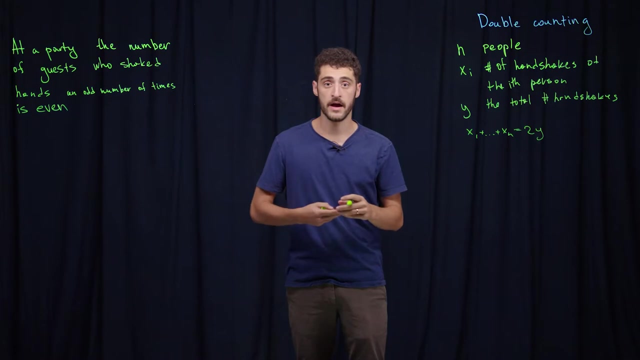 and y be the total number of handshakes. In this case, x1 plus da-da-da plus xn is equal to 2y. just because when we count x1 to xn, we count every handshake twice, as a handshake of the if-person and as a handshake of the jith-person. 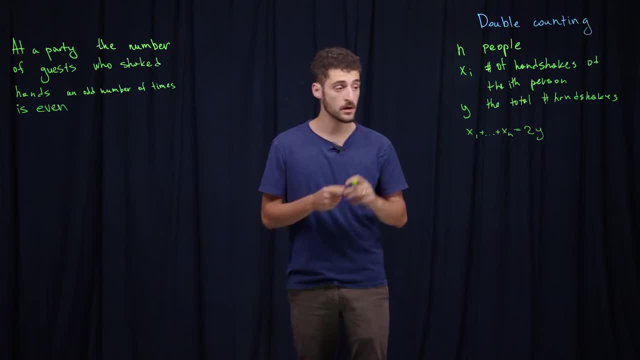 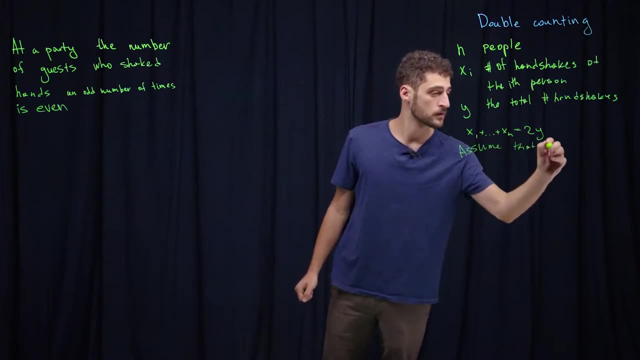 when if-person handshakes with the jith-person. Okay, Assume that the statement we are going to prove is not true, Then x1 plus da-da-da plus xn is odd, because we assume that number of odd xi's is odd. 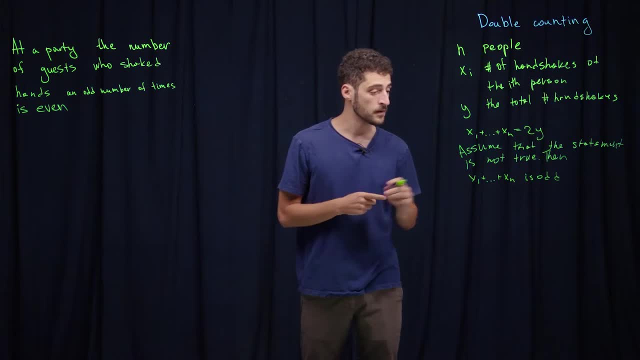 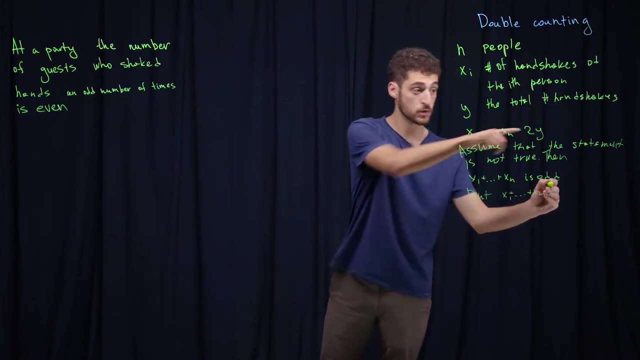 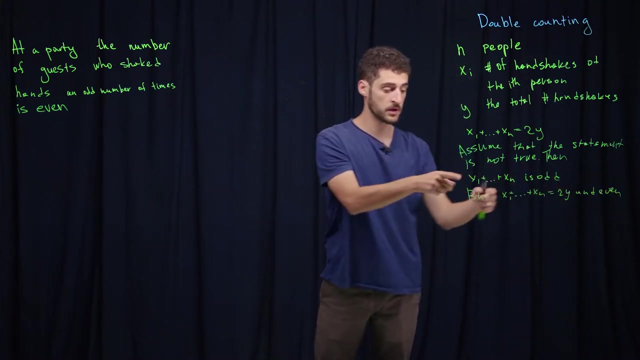 So, when we sum them up, we get an odd number, But x1 to xn is equal to 2y and x1 to xn is equal to 2y And even, which is a contradiction, because we know that it should be odd. 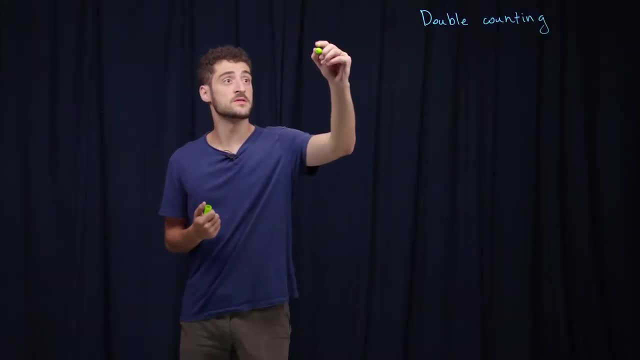 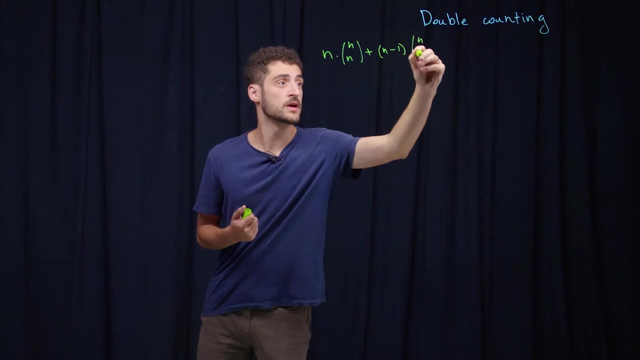 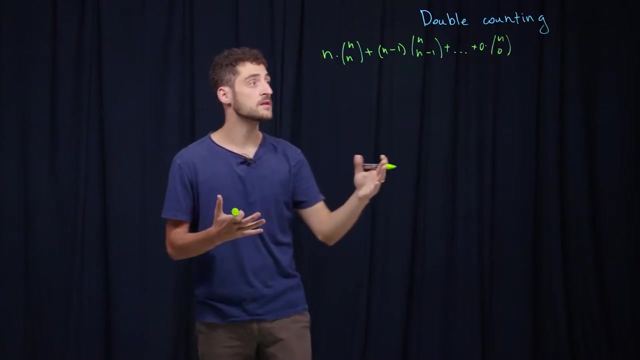 Let us consider another example. So let's consider this: sum n times n. choose n plus n minus 1 times n. choose n minus 1 plus da-da-da plus 0.. So da-da-da plus da-da-da times n, choose n plus n minus 1 times n, choose 0.. 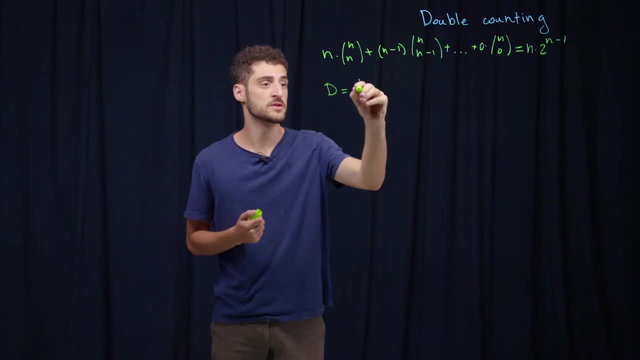 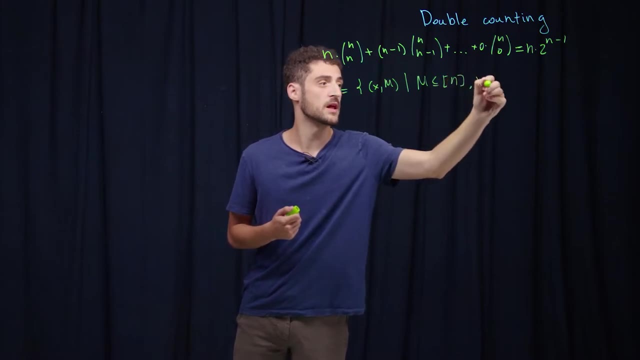 And the statement is that it's equal to n times 2, to the n minus 1.. In order to prove this, consider the set D, which is the set of pairs x- m, where m is a subset of numbers from 1 to n and x is an element of m. 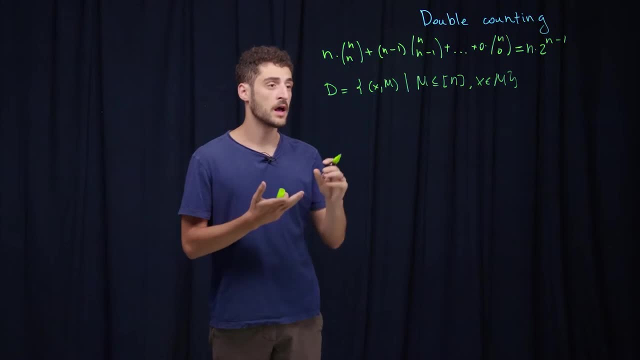 You can think about the set D like this: So you have n people And you need to select some number of them And after that select a two-part of e adults where you know n equals to n raised tier. There are two 30-string sets of 28 as well, but when they don't correspond you have aitude that makes more vam Mapos of that. so when there's no validation, you have annplications. This was the answer for that: 4% for n. 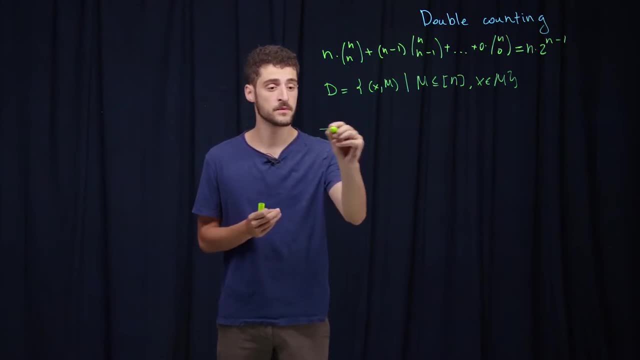 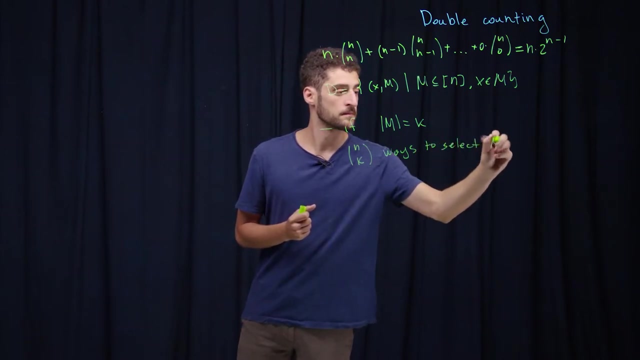 both among them. Note that if the size of m is equal to k, then n choose k ways to select m, k ways to select x. hence, the size of d is equal to n times. n choose n. it's when you have n people. 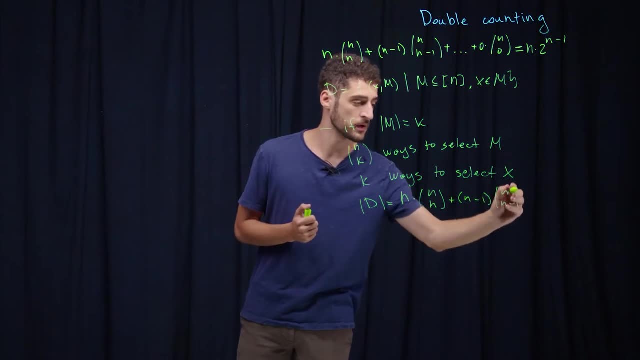 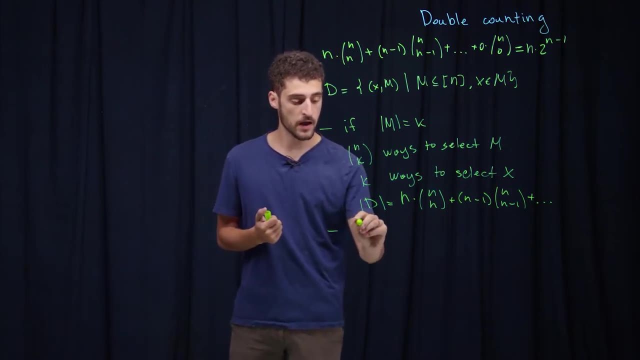 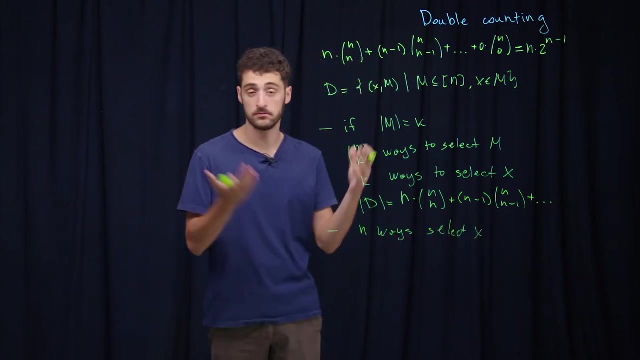 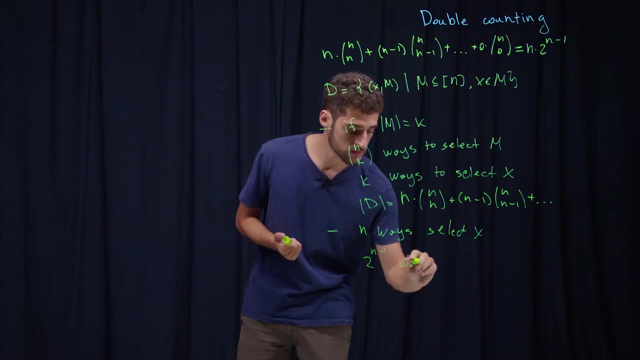 plus n minus 1 times. n choose n minus 1, it's when you have n minus 1 people plus da, da, da. From other point of view, there are n ways to select x, because you have n people, so there are n possible choices, And 2 to the n minus 1 ways to select the rest. 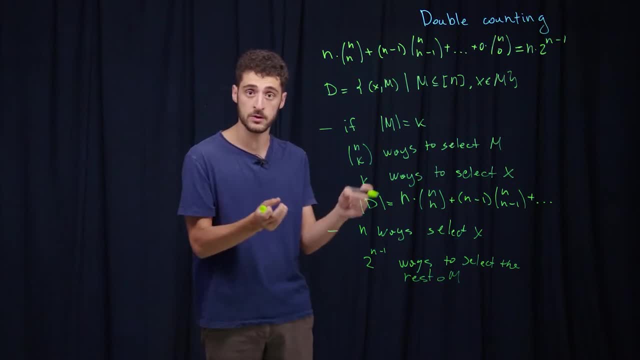 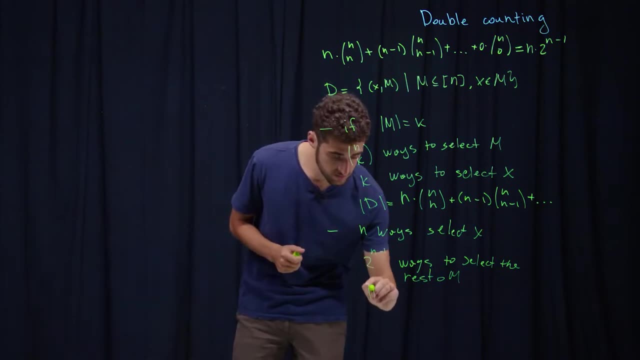 of m, since you already chosen one. so we have n minus 1 elements in the rest and you may choose any of them. Hence the size of d is equal to n times 2, to the n minus 1.. In other words, 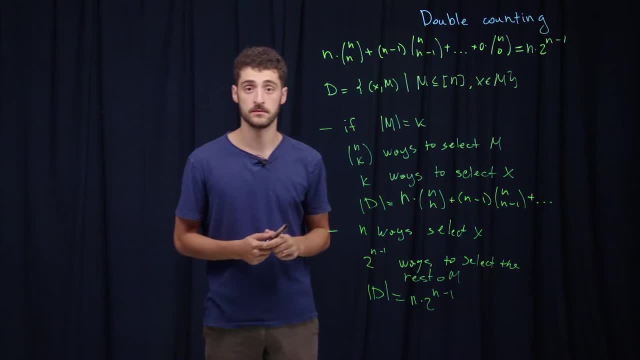 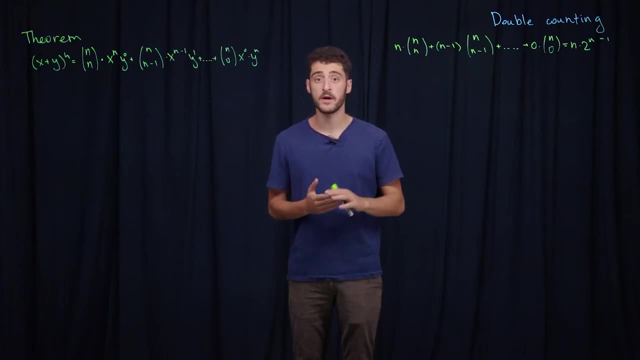 this is equal to this, which finishes the proof of this equality. We may also give an alternative proof of this statement, which is not based on the idea of double counting, but it's quite beautiful and since we are discussing this sum, let's try to give this proof as well. 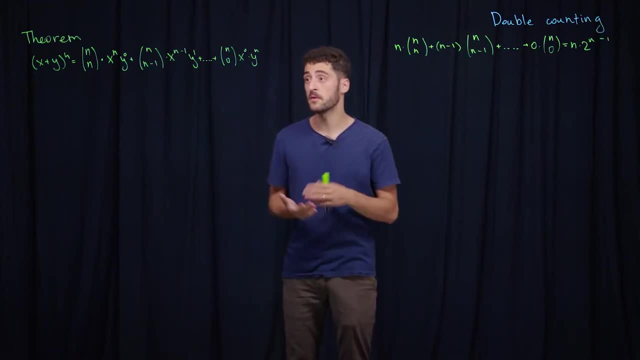 So in the previous lecture we discussed the following equality. It's called the binomial theorem and it states that if you need to compute the value of x plus y to n, you can use the following sum: Now you may notice that this sum is kind of similar to this. 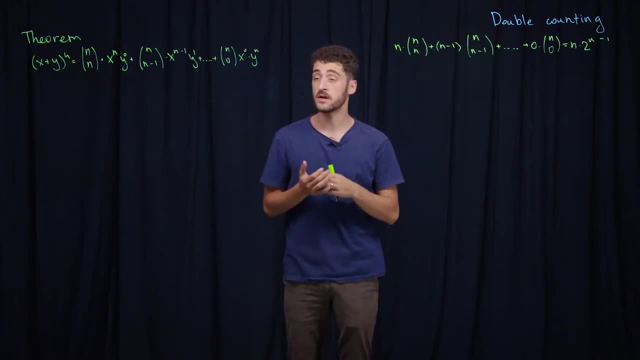 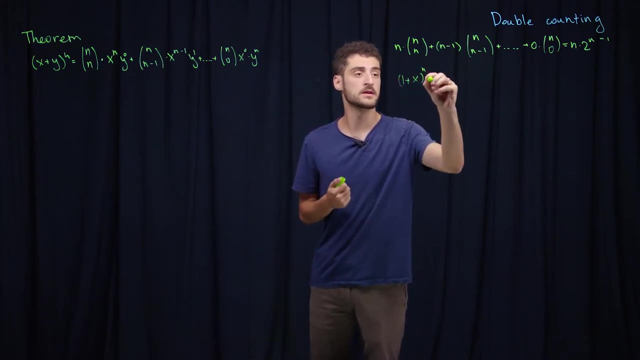 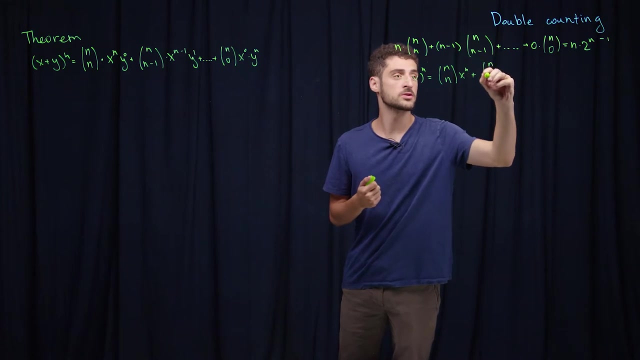 but you have these multipliers here, And so the idea is to use this theorem to get this. Note that 1 plus x to n is equal to n. choose n times x to n plus n. choose n minus 1 times x to n minus 1 plus. da, da, da plus. 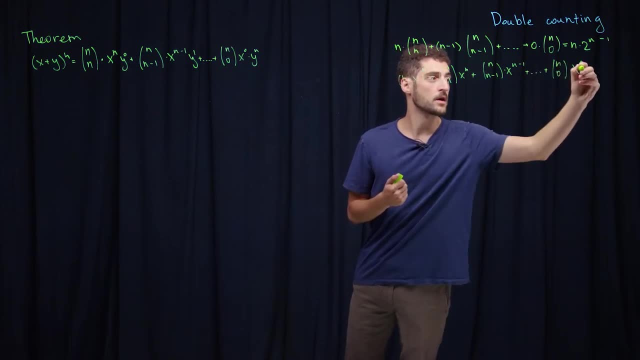 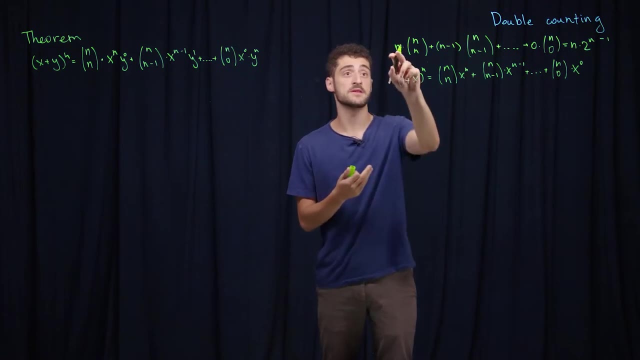 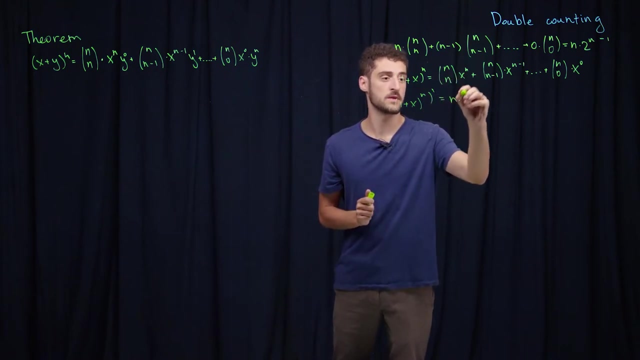 n. choose 0 times x to 0. And okay, it's even closer to this, but still we don't have this. n. n minus 1 and so on. Let's consider a derivative of this. Note that 1 plus x to n. the derivative of it is equal to n time these, so n times n. 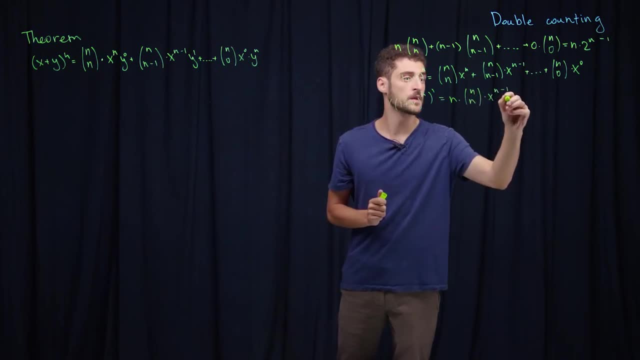 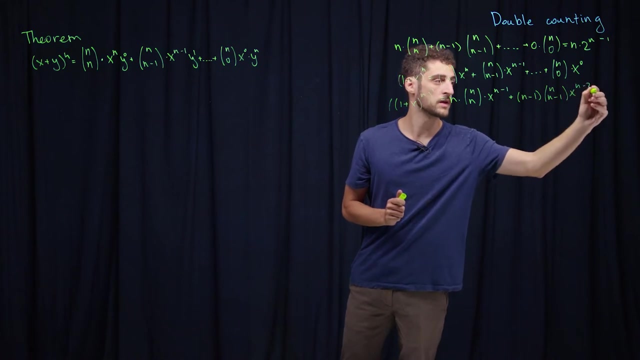 choose n times x to n minus 1, plus the derivative of these, which is n minus 1 times n. choose n minus 1 times x to n minus 2.. So it's n minus 1 times n minus 2.. choose n minus 1 times x to n minus 2, plus da, da da. So now this sum is the. 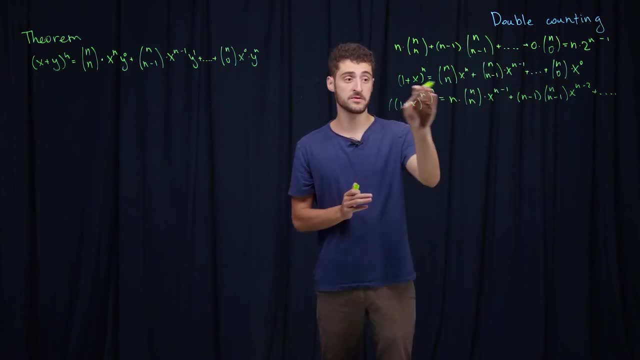 same as this, but with this x, and let's compute the derivative of this: It's equal to n times 1 plus x to n minus 1.. Substitute, let's substitute there, x equal to 1.. This is equal to n times 2 to the n minus 1, because 1 plus x is 2.. 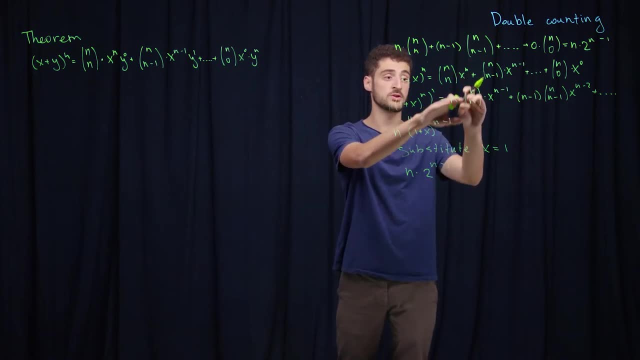 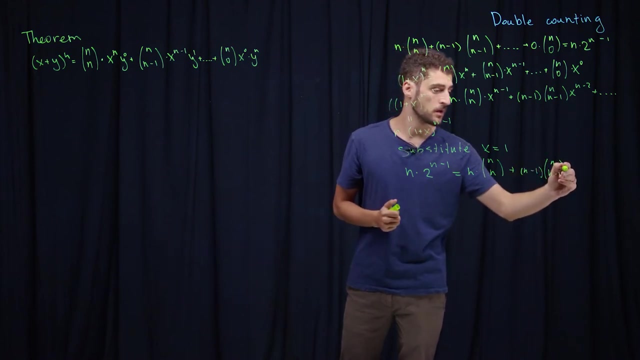 And this one is equal to n times n. choose n times 1 plus n minus 1 times n. choose n minus 1 times 1 to n minus 2, which is 1 plus da da, da. And as a result, we proved the statement we wanted to prove. The last example of the 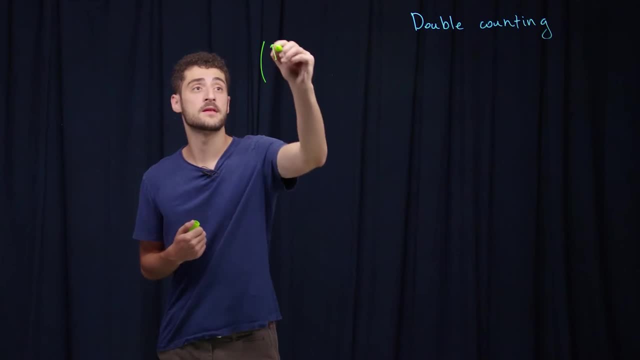 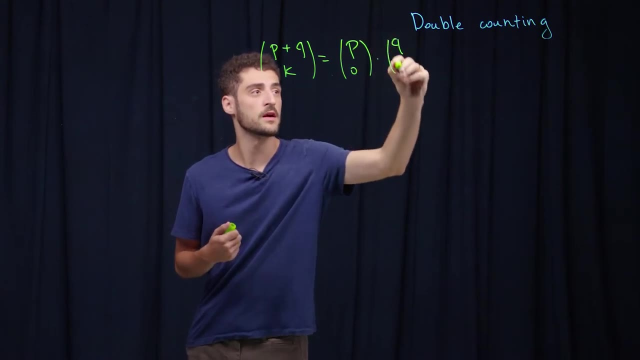 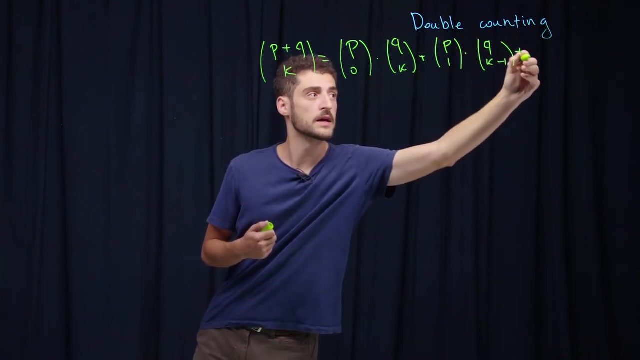 double counting technique is the following. So it states that p plus q- choose k- is equal to p. choose 0 times q. choose k plus p. choose 1 times q. choose k minus 1 plus da, da da. In order to prove this, let's imagine that we have p.